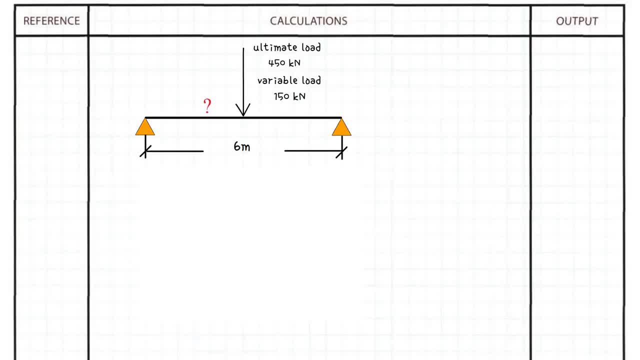 Determine what size of beam is required to support this load, assuming the steel grade to be S-355.. First we need to work out our applied forces. Let's assume beam self-weight is 1.4 kilonewtons per meter. Therefore ultimate distributed load equals 1.35 by 1.4 kilonewtons. 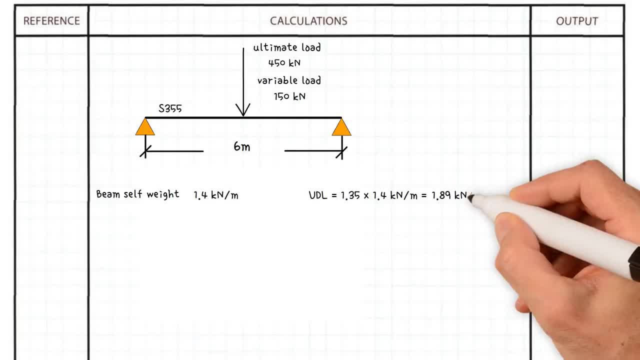 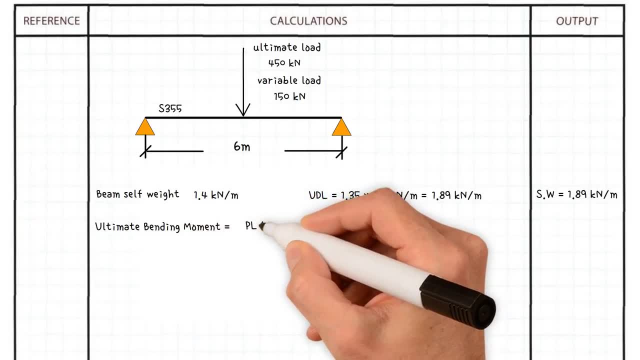 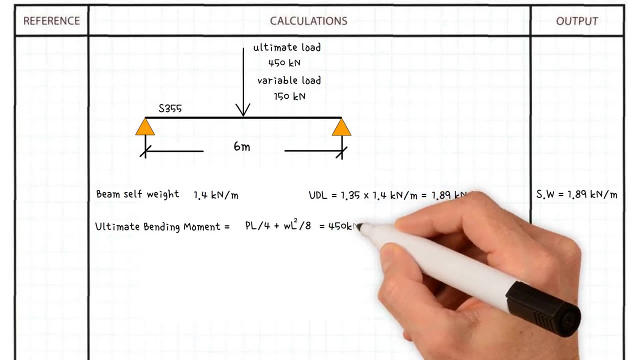 per meter, giving us a value of 1.89 kilonewtons per meter. Next we need to find ultimate bending moment, which equals P times L over 4 plus W l squared over 8, which is 450 kilonewtons times 6 meters over 4. 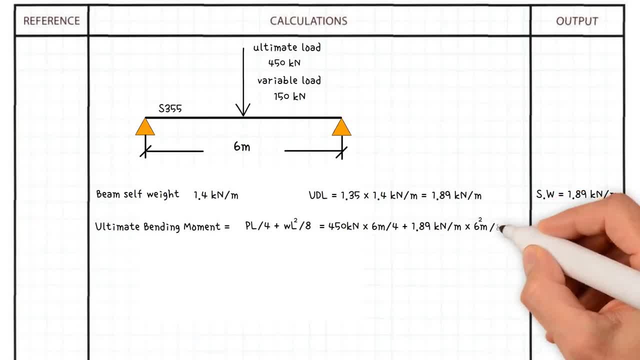 1.89 × 6² over 8. This result in a value of 683.5 kNm. We also need to find out the shear force, which equals 450 kN over 2, plus 1.89 kN. 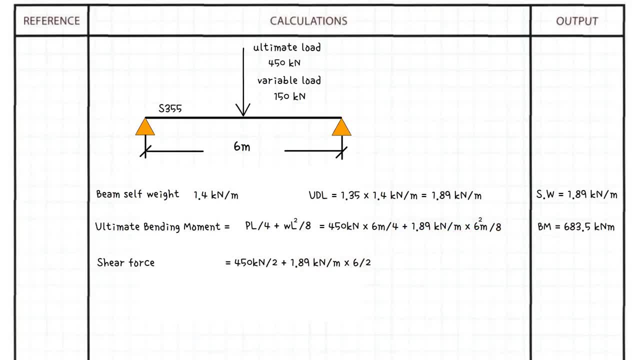 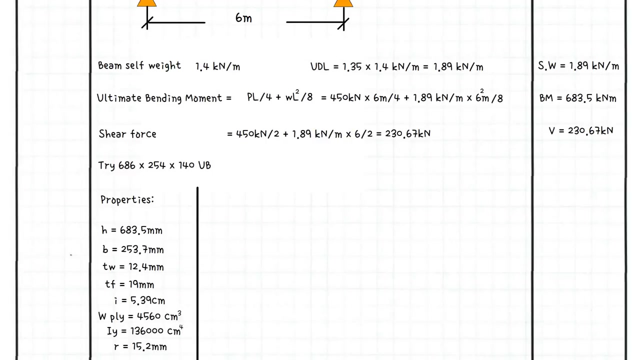 per meter times 6 meters over 2. This corresponds to value of 230.67 kN. Let's try 686 × 254 × 140 UB steel beam, which got the following properties: But first we are required to determine the classification of beam, section: British Standard. 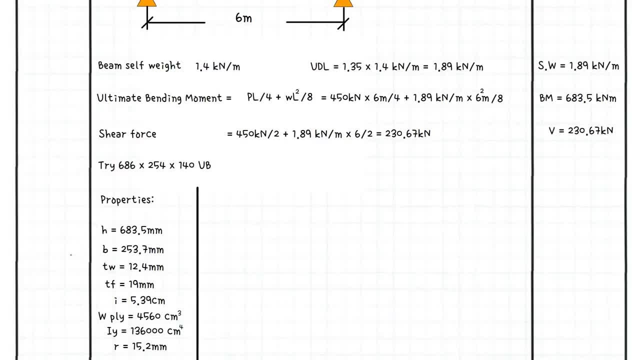 Group's steel beams into four classifications. These classifications are based on a steel beam section's resistance to suffering from a local failure due to buckling. Class 1, plastic: These sections can form a plastic hinge when a bending moment is applied to them without. 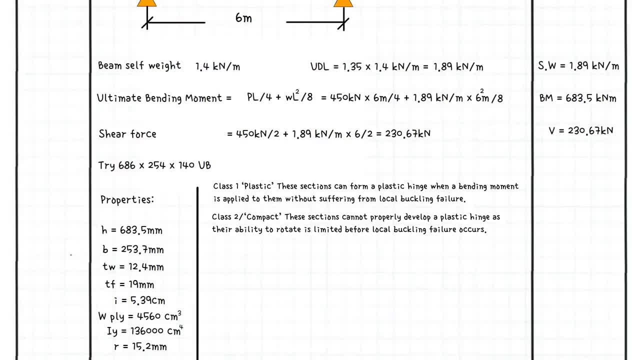 suffering from local buckling failure. Class 2, compact: These sections cannot properly develop a plastic hinge as their ability to rotate is limited before local buckling failure occurs. Class 3, semi-compact: These are sections that can withstand elastic stresses, specifically at the extreme fibers. 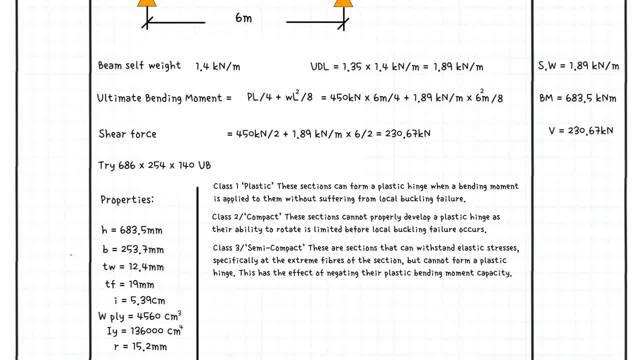 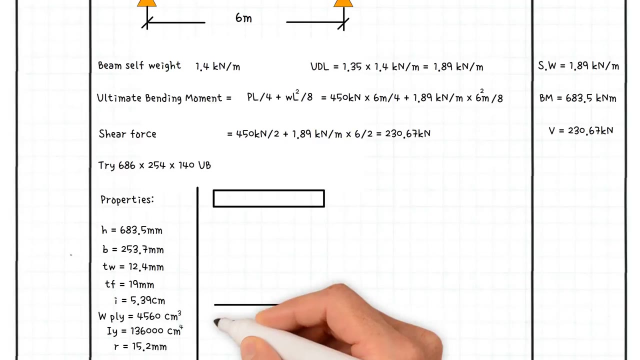 of the section but cannot form a plastic hinge. These sections can used as çaite útilר. In the case of a plastic hinge, these sections are made to be used in a rigid applied multiply series to slightly insecure the metal of the section. This has the effect of negating their plastic-bending moment capacity. Class 4, slender Sections that will fail due to local buckling prior to the point of yield stress. Their plastic bending capacity, therefore, is non-existent When determining the classification of a section, typically two parts of a rolled steel beam. section are considered For a simply supported beam. these are the edge of the top flange and the web, both of which are subjected to slidel energy. The large beam section is USB typebnium, one-pointed, without hot air flow. so this single SLD boundary range 지금. 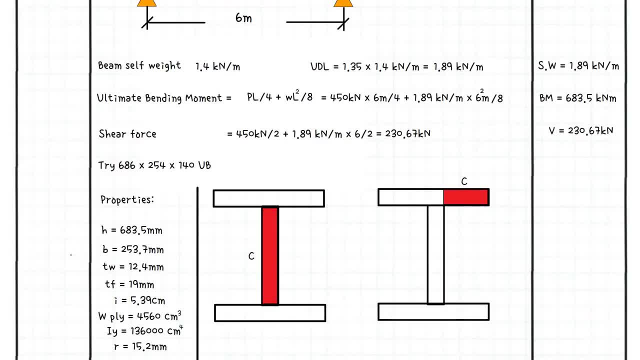 and abombing system is Pres destiny decided which to keep due, not directly but rather sensibly, sozusagen flange and the web, both of which are subjected to compression stress due to bending. table 5.2 in clause 5.5 of bs1993 defines the limits within which the geometry of the elements must lie. 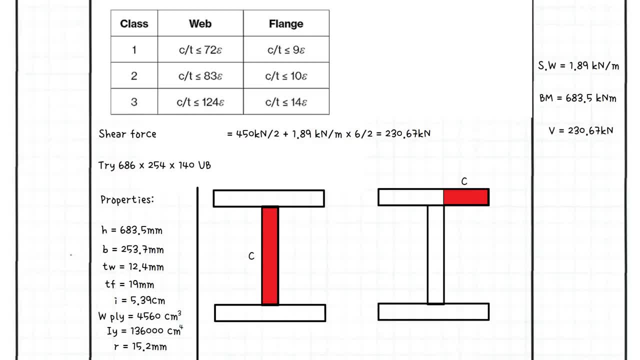 these limits are further modified based on the yield strength of the material. this is defined via coefficient epsilon. the coefficient for section classification epsilon equals the square root of 235 newton per square millimeter divided by the yield strength of the steel based on element thickness. this table indicates the limiting values for various 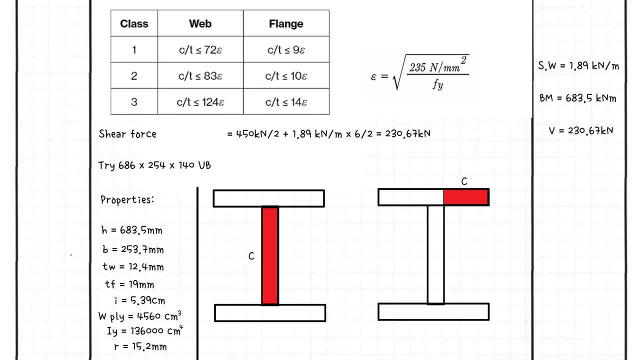 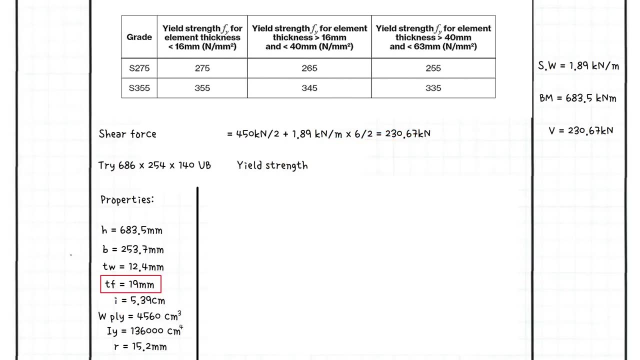 classes of section for both of the elements. if any of the ratios go beyond those stated in this table, the section is considered to be in the class 4 category. so now back to our worked example. the yield strength for element greater than 16 millimeters and less than 40 millimeters is 345 newton per square millimeter. for steel grade of s 355. 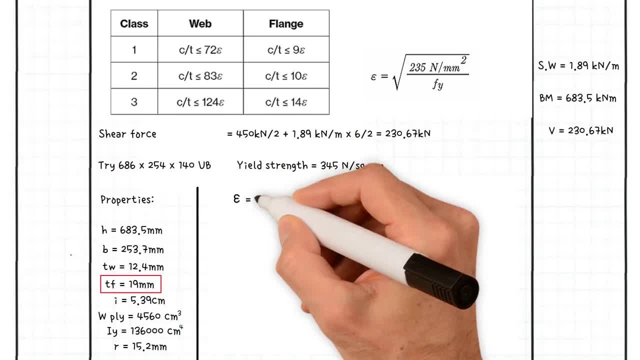 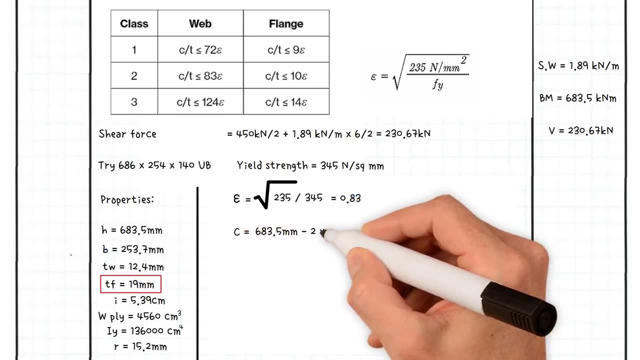 therefore, coefficient epsilon equals the square root of 235 divided by 345. this gives us a value of 0.83. working our c web, which equals depth of the section minus two times the thickness of the flange, minus two times the root radius, this gives us a value of 615.2 millimeters. this gives us a value of 615.1 millimeters. 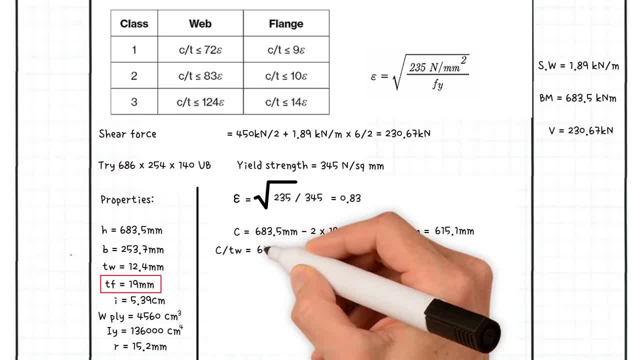 as a result, c over web thickness equals 615.1 millimeters over 12.4, which is 49.6. we compare this to 72 epsilon, which equals 59.4, which is greater than 49.6. therefore, the section is plastic class one. 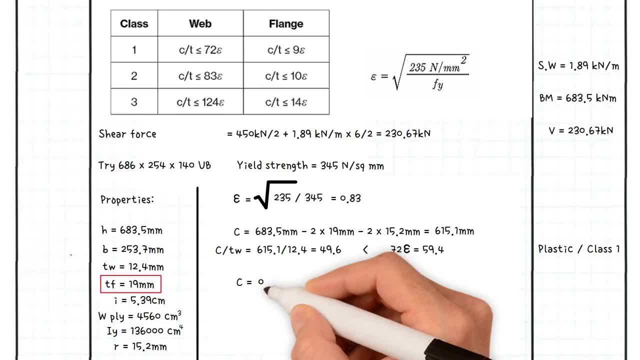 next working our c flange, which equals half of the width of the section, half of 253.7, minus half of web thickness, 0.5 times 12.4 minus the root radius, 15.2 millimeters. this gives us a value of 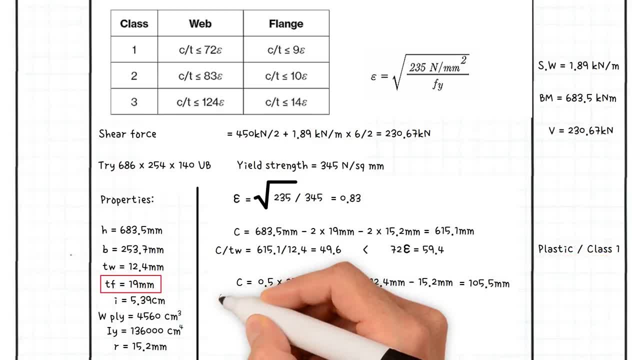 105.5 millimeters. as a result, c over flange thickness equals 105.5 millimeters divided by 19 millimeters, which equals 5.55. we compare this to 9 epsilon, which equals 7.43, which is greater than 5.55. 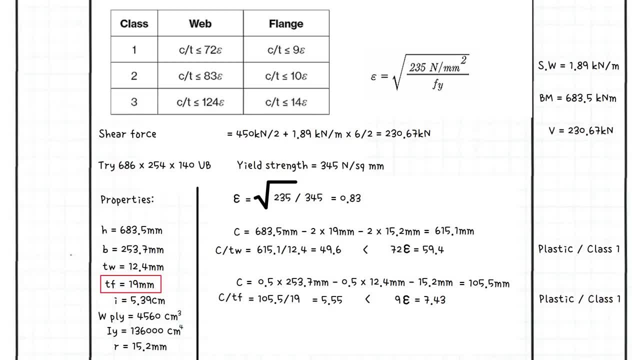 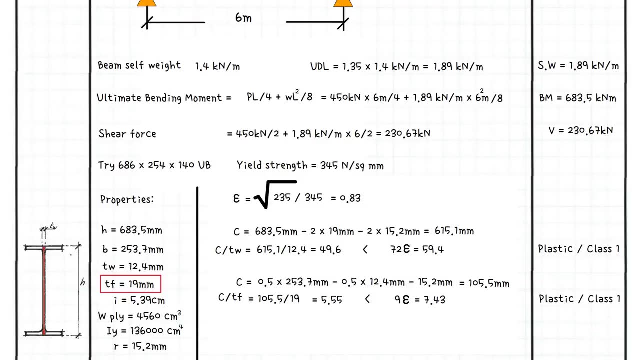 so the section is plastic class 1. therefore, section is class 1 category. next we need to check the shear resistance. in the case of class 1 and 2, rolled steel beams, the design shear resistance is the cross-section area of the part of the beam that is resisting shear. 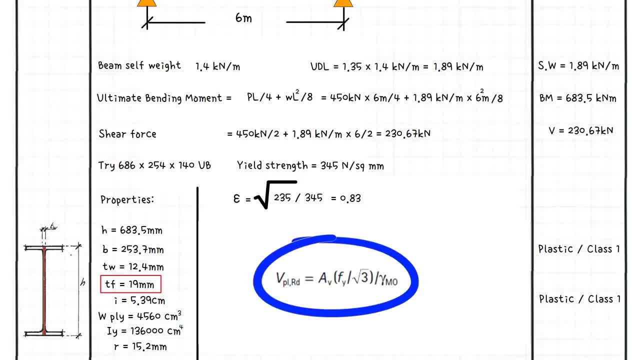 is the cross-sectional area of the web and the thickness of the flange times the yield strength of the steel divided by the square root of 3, divided by the partial factor for the resistance of cross-sections, which in the UK is set at 1.. 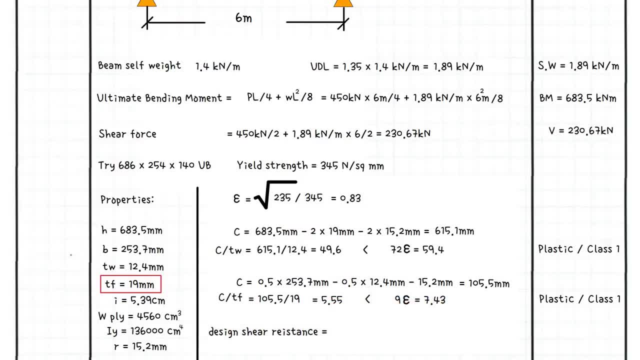 Therefore, the design shear resistance equals: depth of the beam: 683.5, times web thickness, 12.4 mm. times the yield strength of the steel: 345, divided by the square root of 3, divided by 1000 to convert to kilonewton. 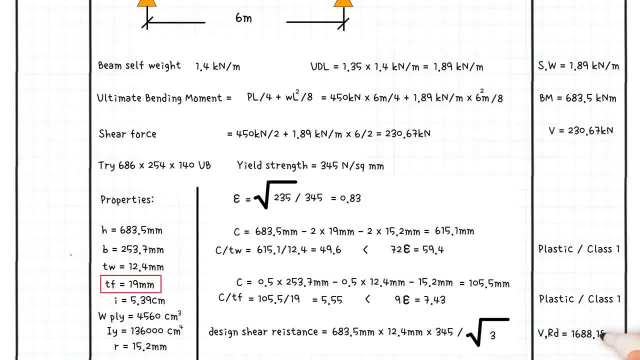 This gives us a value of 1688.18 kilonewtons, which is greater than applied shear 230.67 kilonewtons. Therefore, the shear resistance of section is acceptable. Check for bending Moment resistance modification factor due to high shear. 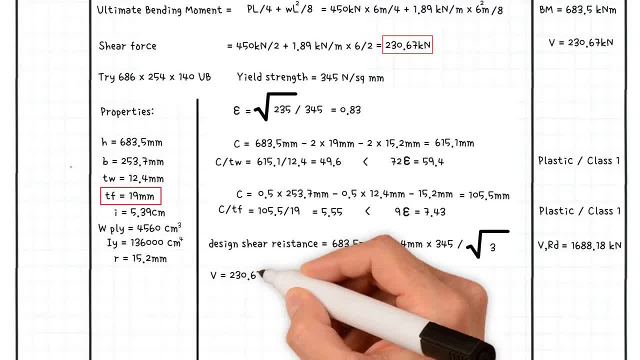 Applied shear force 230.67 kilonewtons is less than half of the design shear resistance 1688.18 kilonewtons. Therefore, no reduction in bending resistance. Moreover, we need to check the section bending moment resistance. 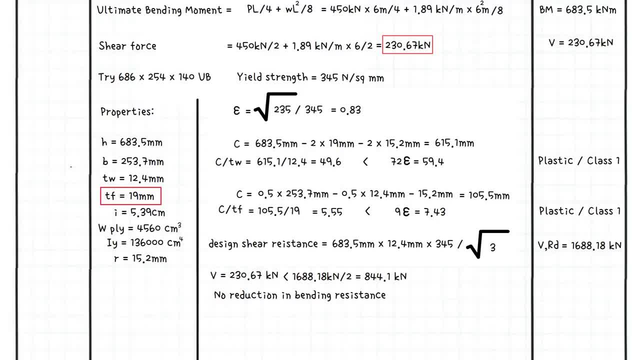 In the case of an unrestrained portion of a beam, a factor is applied to the bending moment. resistance P 1688.18 kilonewtons. S-355 grade steel non-dimensional slenderness. λ equals the distance between restraints to. 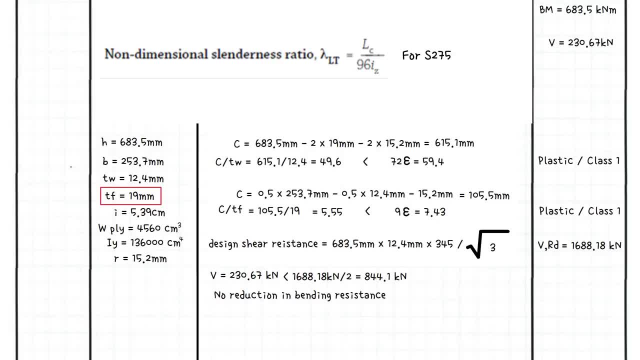 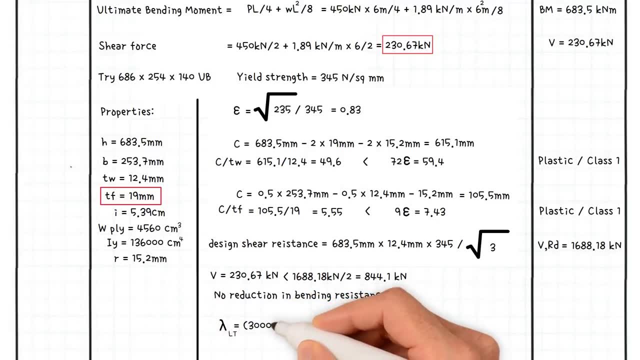 the compression flange of the beam, divided by the radius of gyration about the minor axis of the beam, divided by 85.. Which equals 3000 mm divided by 53.9 mm, divided by 85. This result in a value of 0.655.. As the non-dimensional slenderness is established, the value of 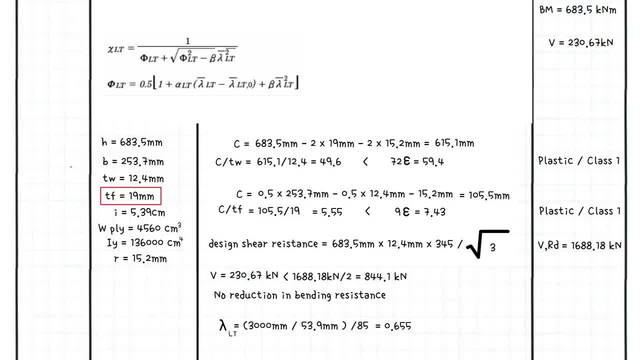 reduction factor σLT, determined using equation 6.57 of clause 6.323 of BS 1993.. αLT is the imperfection factor and is found in table 6.3 of BS 1993, which reads against the: 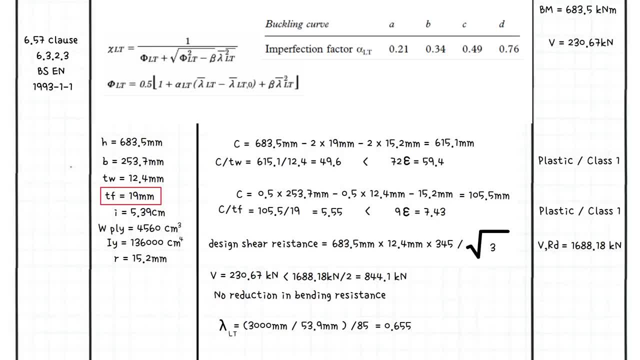 steel beam's buckling curve. The buckling curves are labelled A to D and can be found in Clause National Annex 2.17.. The buckling curve is dependent upon the H-B ratio of the beam section. The value of β and λ are defined as 0.75 and 0.4 respectively. Depth of the beam: 683.5 mm, divided by 253.7 mm, equals 2.7.. Therefore, curve C applies. As a result, the imperfection factor α equals 0.49.. Putting these numbers into our equation, then the reduction factor would be equal to 0.853.. 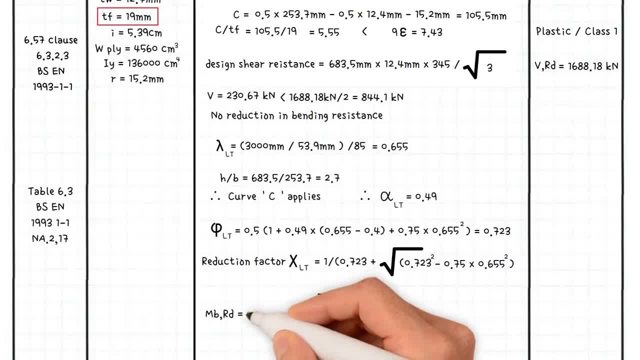 Consequently, the bending moment resistance equals the reduction factor 0.853, times the major axis. section modulus of the beam based on its classification, which is plastic. section modulus for class 1 or 2, which is 4560 times 10 the power of 3 millimeters cubed times the yield strength of.